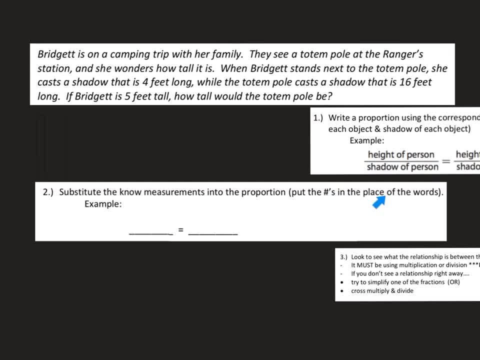 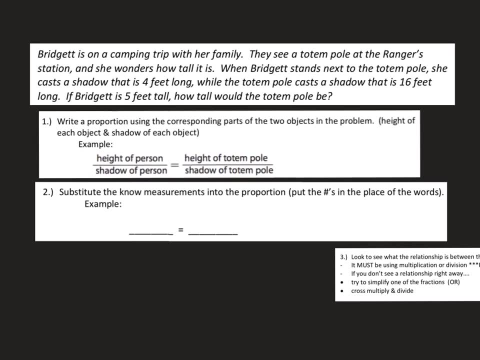 proportions. So basically, I'm putting the numbers in place of where the words went. If I pull this one back out, so I can see it at the same time. Okay, so we have person height on top When we go look up in the story problem the person's height. 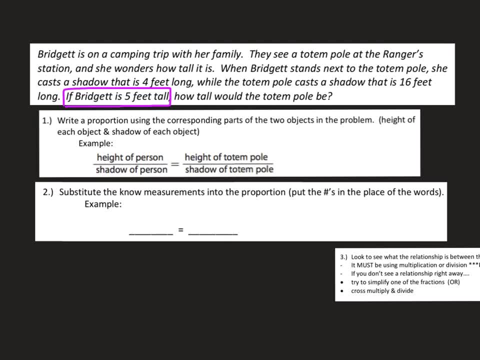 it says Bridget is five feet tall. So then I would put five and this is how tall she is, And underneath that it says: I need the shadow for the person. When we read back up in the top the shadow, it says: 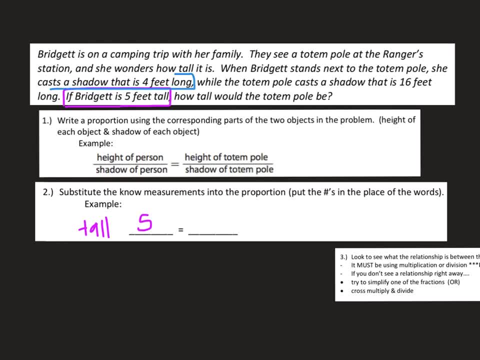 that she casts a shadow that's four feet long, And then the word she is over here, So I'm going to put four, And then this is her shadow. The second ratio over here should be about the totem pole, And then again we're going to say how tall it is, and then the shadow on bottom. When you look back in the story, 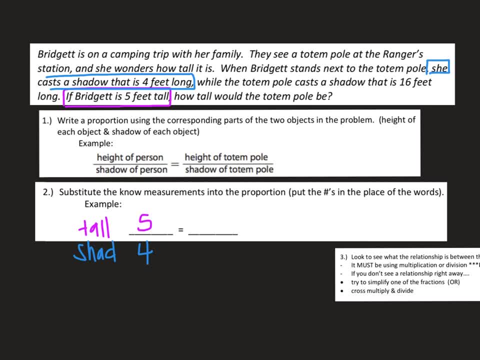 problem. it says that the totem's pole is four feet long, So I'm going to put four. And then this is her little shadow. The shadow is 16 feet. The shadow went on the bottom, So I'm going to put 16.. And we don't. 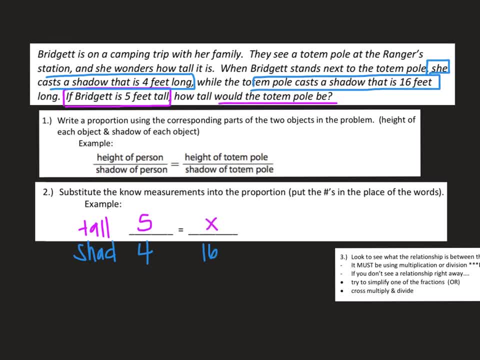 know how tall would the totem pole be? You can put any variable you want there, or an X, or a question mark, It doesn't matter. What I'm going to do is I have a third tab over here and it says that I want to. 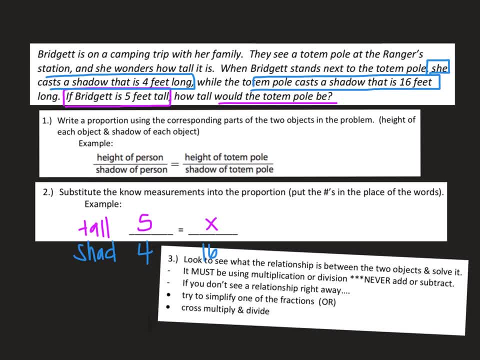 try to look at the relationship between the two objects And I always want it to be through multiplication or division. Multiplication: never add or subtract. Okay, It also says you can try to simplify the fractions. right here. Simplify the fractions, Or if you don't know what number is going to go in the missing spot, you can always cross. 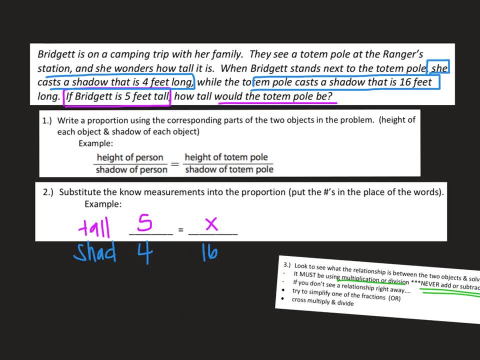 multiply and then divide. I'm going to scoot that one back out of the way, Because for me, I'm going to try to find out what number is going to go in the missing spot. Okay, So for this example, we can tell what's. 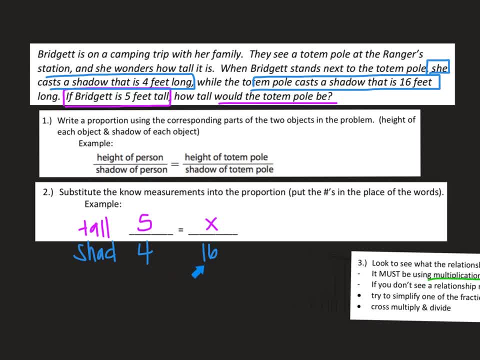 happening. The shadow of the person compared to the shadow of the totem pole. This has a perfect relationship. This is being multiplied by four. The totem pole's shadow is four times longer than hers, So that means that the height of the totem pole should also be four times taller than what she is. 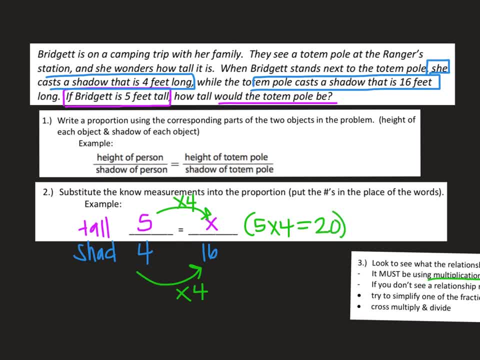 Okay. Therefore, the totem pole should be four times taller than what she is. So that means that the totem pole should be 20 feet tall. Another thing you could do: if you're a picture person and you wanted to do this, you could draw. 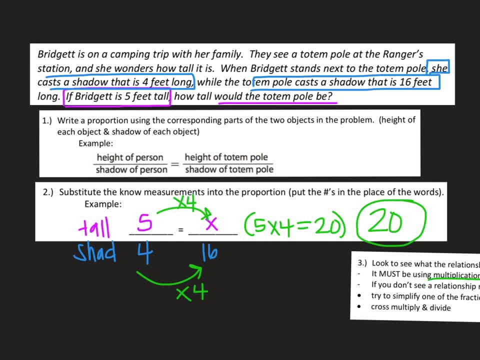 this is the girl And you could have this labeled. She's five foot tall and her shadow is four times taller than hers- Another thing you could do. if you're a picture person and you wanted to do this, you could draw. this is the girl And you could have this labeled. She's five foot tall and her shadow is four times taller than hers. 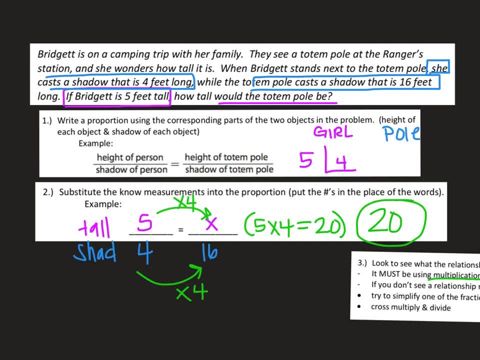 Another thing you could do. if you're a picture person and you wanted to do this, you could draw. this is the girl And you called her elf, but that's not what this was for. Next, you could head to your financial aid. In months or months, you could get really. niveled. Number one is four. The world is doing pretty well right now. Number two is for the totem pole. The hundred plus five is very nice, And then you could have the totem pole and also just do the same measurements. We only know that the shadow is. 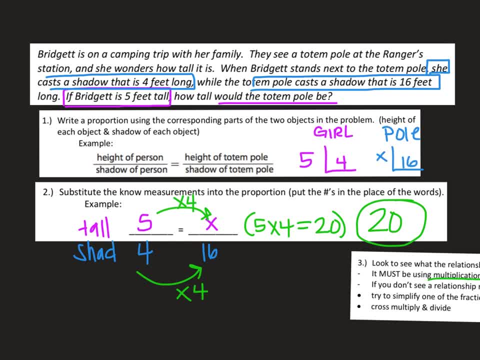 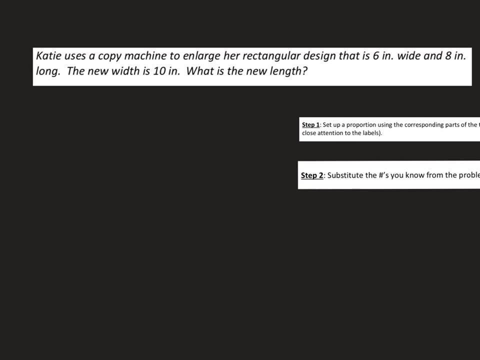 speak utn 16, and we don't know the height. thatmuş κ Realني sketches, but draw the lines representing the height and the shadow. all right, this second example, this one's really short. Katie uses a copy machine to enlarge her rectangular design that is six inches wide and eight inches long. the new width. 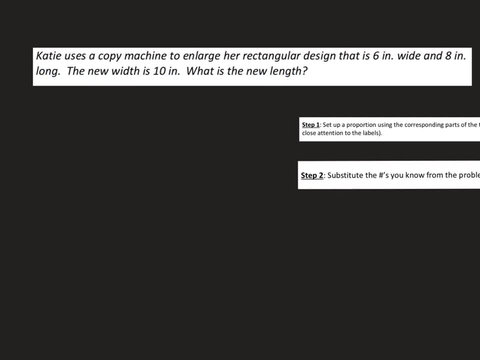 is 10. what is the new length? okay, for this example, I'm going to draw the pictures. so she has a rectangular design. okay, this is the original and the measurements for the original. one is 6 inches wide and 8 inches long, so I'm gonna put my 8 down here, because that's. 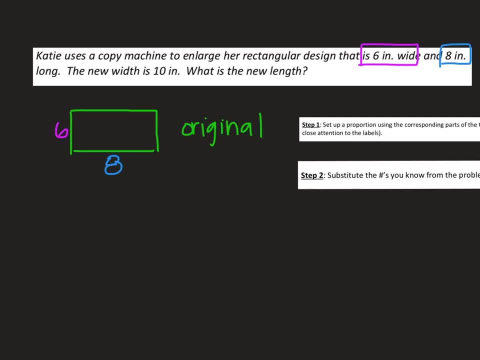 a longer piece And then 6 on the side for the width. Now, when I get ready to make my new picture, it's not the same size. She has enlarged it because it says so in the story. She's going to enlarge it. 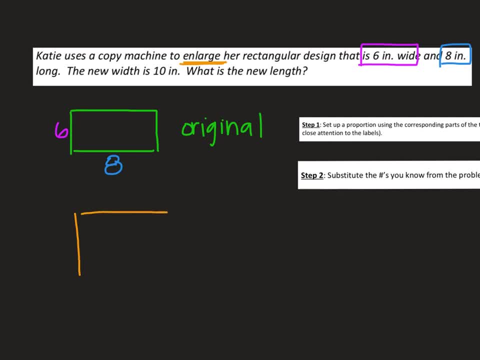 So I'm going to make a larger rectangle And then I'm going to put in the dimension. This one says that it's the width that you know, And it says that the width is 10.. So I would put a 10 right here. 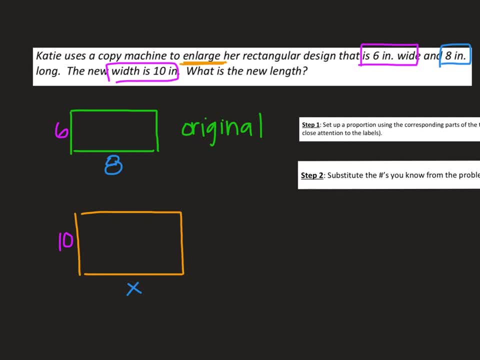 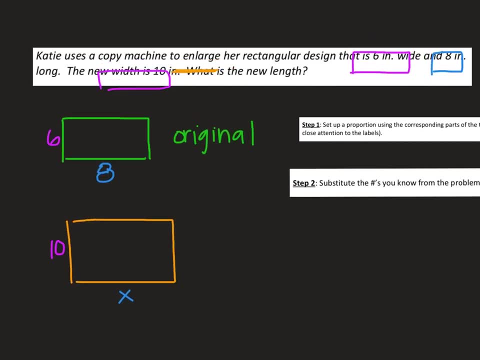 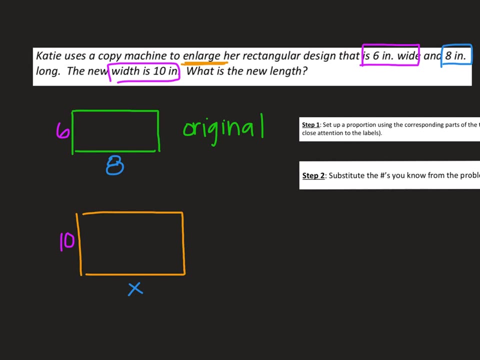 And then we don't know what the length is. Again from the last slide. Whoops, Oh, that's not going to work. Okay, from the last slide, what we were saying was: set up a proportion And then see if you can determine the relationship. 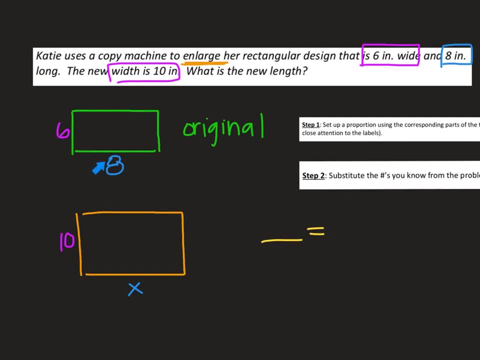 I'm going to take these two, the numbers for the original, 6 inches wide and 8 inches long, And I'm going to set that up 6 and 8. And that's going to be equal to my new proportion, or my new shape is going to be 10 by X. 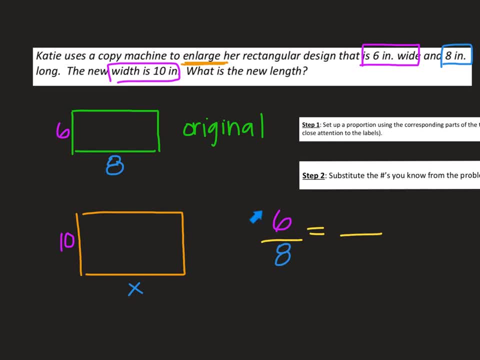 Okay. So if you can see the way I've color coded these, I'm putting the pink number or the width on top and then the length on bottom. So 10 needs to go on top for me and X needs to go on bottom. 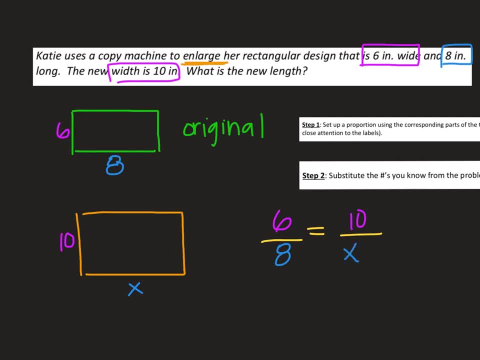 10 and X. I really like color coding because it just makes it easy for me. But if you're fine, not color coding, it's totally okay. This particular example, I'm going to go with the cross: multiply and divide method. 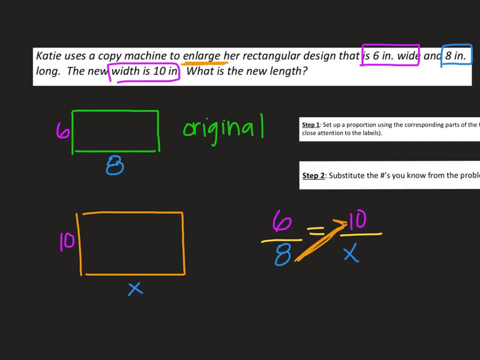 Okay, 8 times 10.. 8 times 10 is 80. And then, when you're done, you need to divide by 6.. So 80 divided by 6. That is going to be 13.3. repeating: